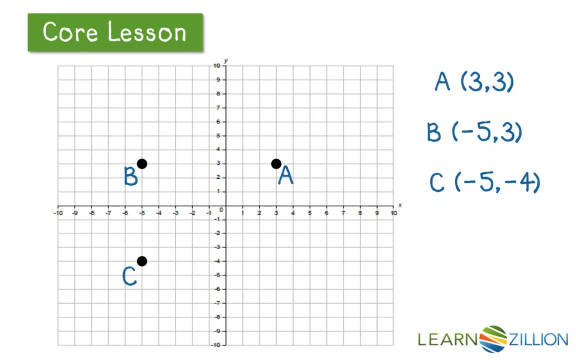 so movement on the y- and x-axis. Now I'm trying to find the fourth vertex. These are three vertices of a rectangle and I want to find the fourth vertex of this rectangle. Now, the way that I'm going to do that is I'm going to find the opposite location of the points on this coordinate plane. 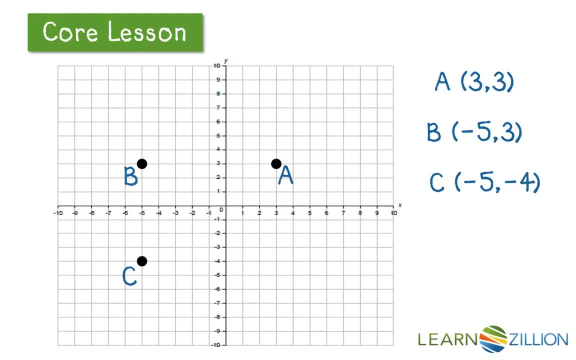 points on this coordinate plane. Now what I'll do is I can see that the fourth vertex would be a positive x value and a negative y value. So what I'll do is I'll use the same value in the coordinate pair of A, which is a 3, and I'm going to 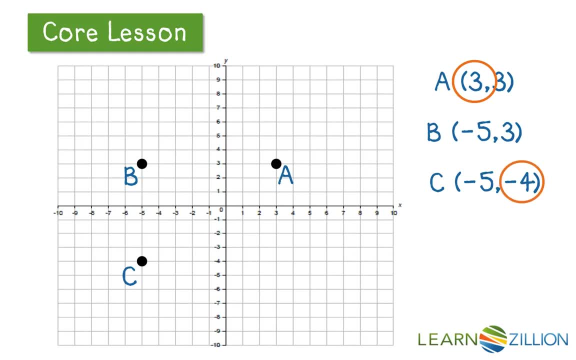 use the negative value of C, So I'm going to create my own new ordered pair at 3 negative 4.. Now that looks like a rectangle, but I want to make sure. So what I can do is I can look at the distances between these points and I can. 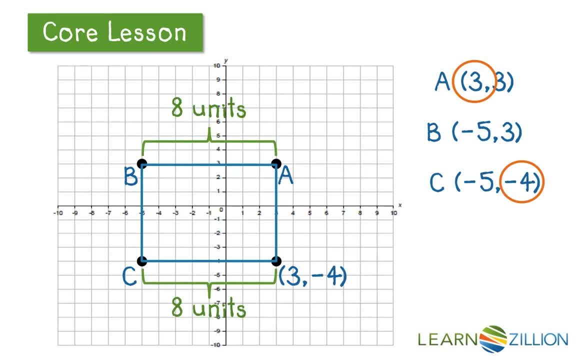 see that the distance between A and B and C and our new fourth point is 8 units and the width would be 7 units. I can see that I've actually created a rectangle and the fourth point that I was looking for to finish the rectangle. 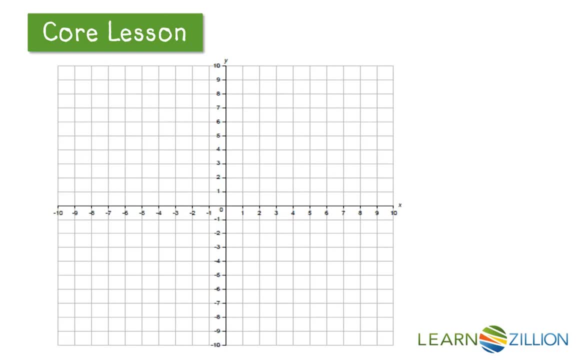 was 3 negative 4.. At the beginning of the rectangle, I've actually created a rectangle and I've I asked us how we could find the fourth vertex of a rectangle. Here were the points that I showed you at the beginning. We had 7, 4, negative 2, 4, and we 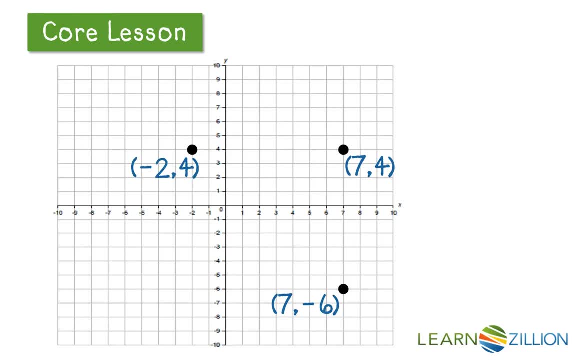 had 7, negative 6.. Now I'm trying to find that last vertex. I can see that it's going to be opposite of negative 2, 4 and opposite of 7, negative 6.. So the x value has to be a negative number and the y value has to be a negative number. 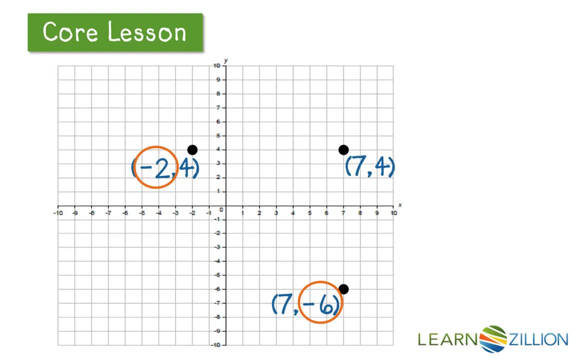 So the fourth and final point that I need to finish: my rectangle is at negative 2, negative 6, and I can see that this creates a rectangle. Now, the length of the rectangle is 9 units and the width is 10 units, so I can prove that. 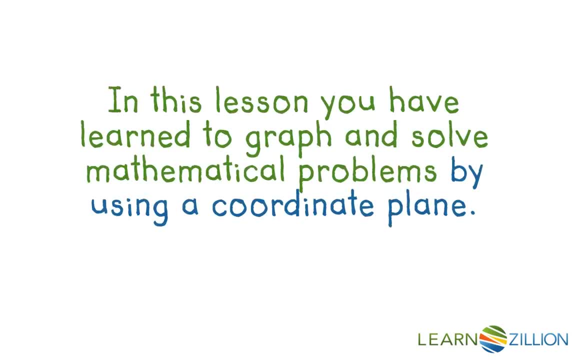 it is actually a rectangle. In this lesson you have learned to graph and solve mathematical problems by using a coordinate plane.